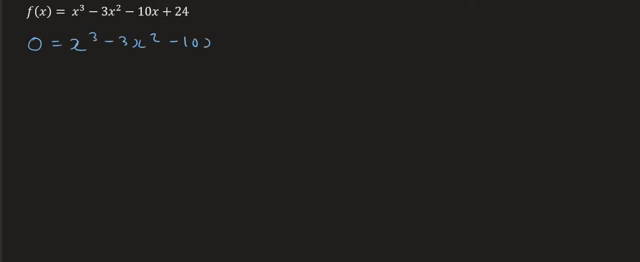 So let's do that and let's just make sure I write everything down correctly, unlike in my previous lesson. Now what we do is we find the first value by plugging in random numbers on the calculator. Now the numbers that you should try would be minus 3,, minus 2,, minus 1,, 1,, 2, and 3.. 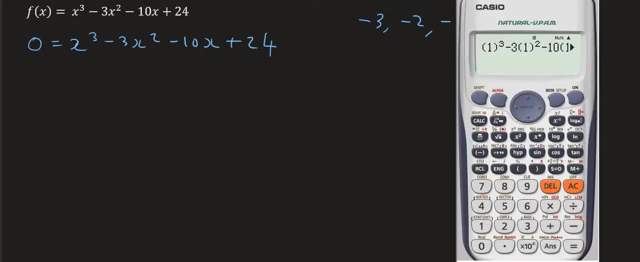 So I'm going to start by plugging 1 into the place of x, like that over there. So you see, wherever I've seen an x, I've used a bracket and I've plugged in a 1.. I'm then going to say equals and I get 12.. 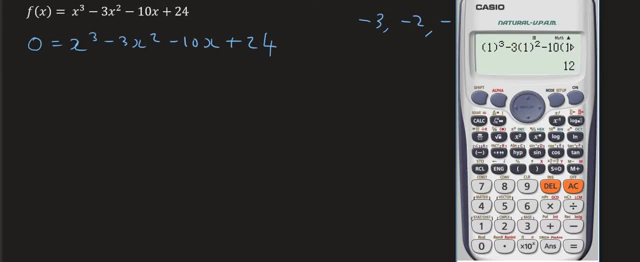 That's not what I'm looking for. I would like the answer to be zero. So then I try the next value. So I'm going to try 2.. So you see, wherever I see an x now, I've replaced it with the number 2.. 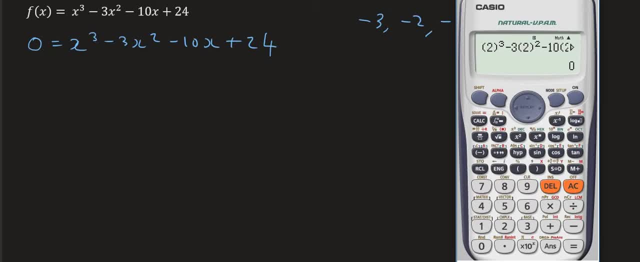 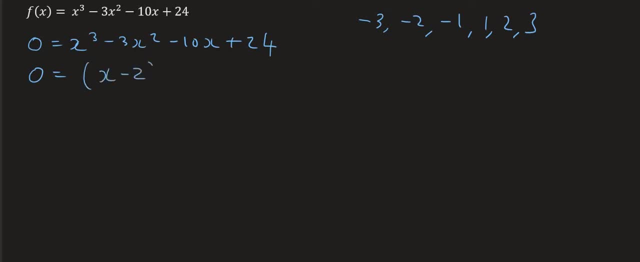 Aha, and there I get a zero. So that's good. That's the first step of this technique, And so what we must remember, though, is that if x is 2, then in bracket form it must say x minus 2.. 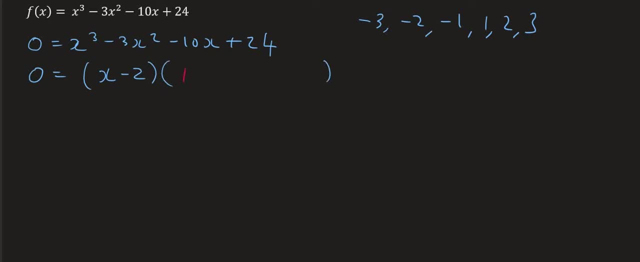 Then remember. what we're left with here is some type of trinomial. We don't know what the letters are, so we'll just say a, b and c. Now, a and c are the easiest to find at this moment in time. 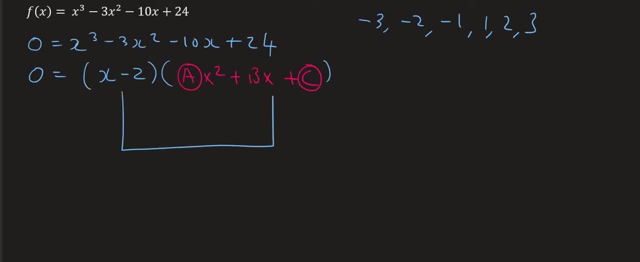 The reason is the following: If you had to multiply these two brackets together, where would you get x to the power of 3?? Well, it would only happen in one place. I'm going to say here one place, That's when you multiply this one and this one. 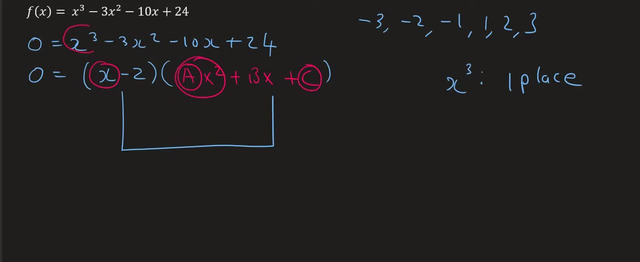 So that times that should give us x to the power of 3.. So that means a will have to have a value of 1.. Because have a look here now: If I had to multiply these two together, that would give me x to the power of 3,. 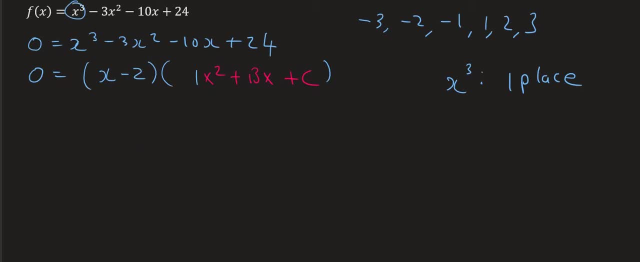 and that's exactly what we had over there. The next one you should look at is this over here. So where, if you had to multiply these two brackets together, where would you get a constant? Now, remember, a constant is a number that does not have an x with it. 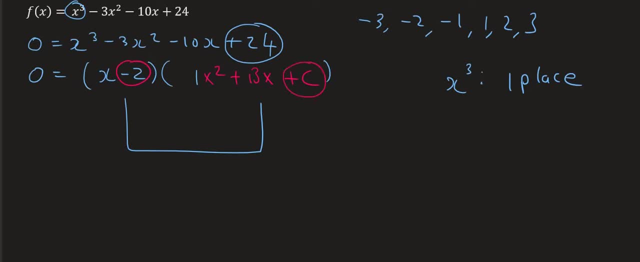 That would be when you multiply this number and this number. Now we would like that answer to be 24.. That means that c should be negative 12.. Because if we now had to multiply those together, you would have minus 2 times by negative 12, which would give us 24.. 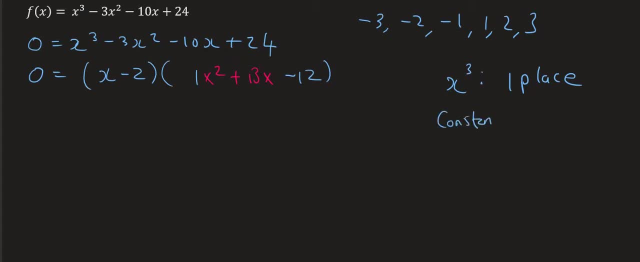 So, with the constant- so I'm just going to say constant- how many places did we have to look at? Only one place, And that helped us to find a, The first one that helped us to find c. Now we've got to find b. 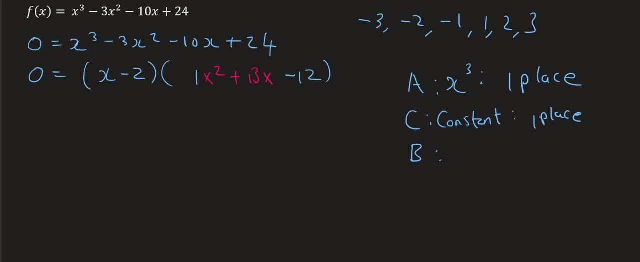 Now, this is the more complicated one, So what you need to do is choose either the x squares or the x's. In the previous lesson, I chose the x squares, So to change things up a bit, I'm going to choose the x's this time. 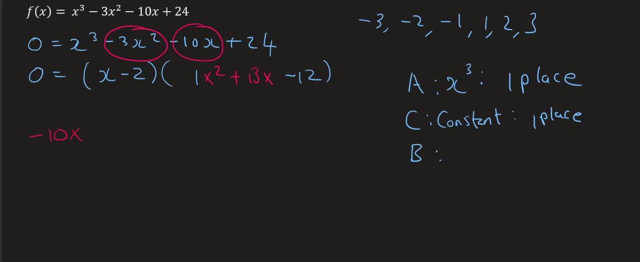 So I know that the answer should be minus minus 10x. Now where would you get an x if you had to multiply these two brackets? Well, this is going to happen in two places. okay, And that's the big difference. is that for a and for c? 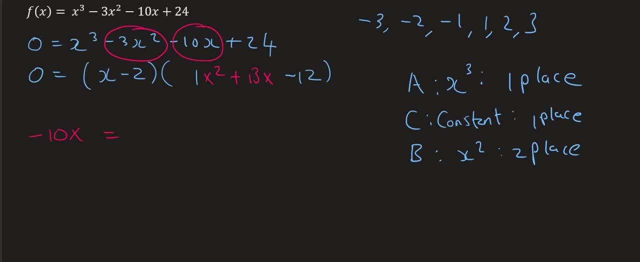 there was only one place where it happened, But for b it happens twice. Have a look here. I could multiply those two together. That would give me an x squared. And I could also multiply those two together, And that would also give me an x squared. 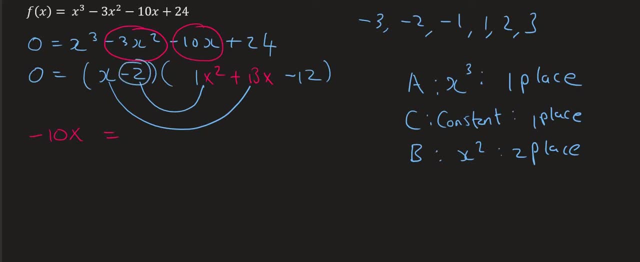 So all I do is I form an equation. So when I take minus 2 and I multiply, multiply it with x squared, that gives me minus 2.. Oh, but Kevin, we said we're going to use the x's, not the x squares. 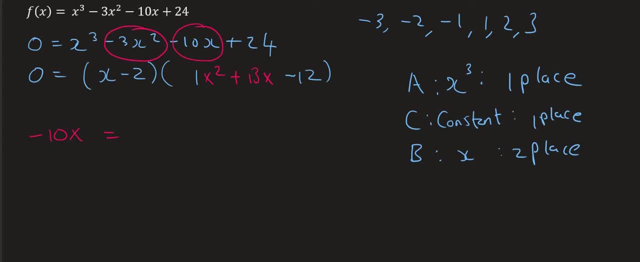 Okay, sorry guys. Nonetheless it's still going to happen twice. So it will happen when you multiply those two together and those two together. So minus 10x will be equal to well. that outside line is going to be x times by minus 12.. 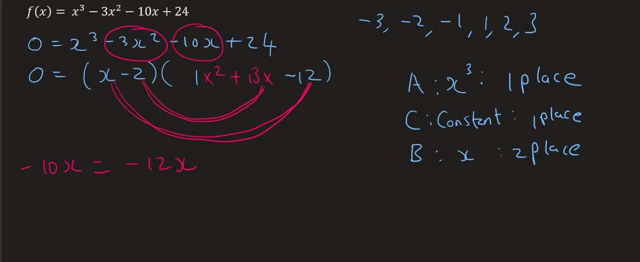 Well, that's minus 12x, And then the inner one is going to be minus 2 times b, which is minus 2bx. Then we can we can ignore the x's and we can have: minus 10 equals to minus 12 minus 2b. 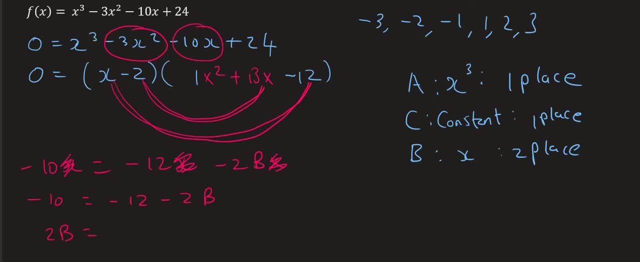 I'm going to take the 2b over to the left And then on the right. we're going to end up with negative 2, because it will be minus 12 plus 10.. And so b is going to be equal to negative 1.. 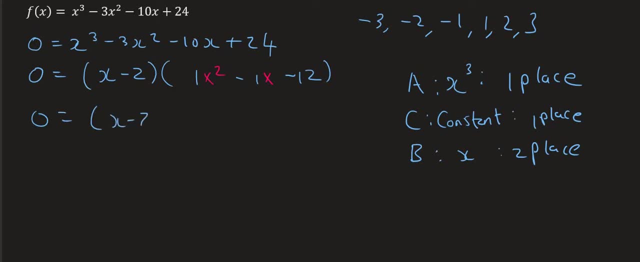 And so there we have it Now. if possible, you would want to. you would want to factorize out the second bracket into two smaller brackets. This one's going to work quite nicely: It's x minus 4 and x plus 3..